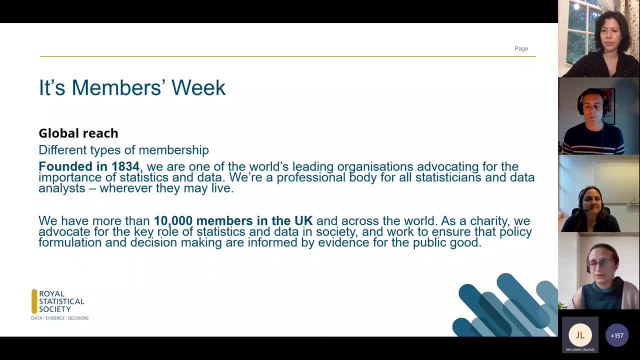 we are a professional body of statisticians from different creeds, be it here you know, theoretical statisticians, applied statisticians in every, from different disciplines as well, and data analysis and in we are in fact global. we have a global reach. a quarter of our membership, ten thousand membership, is from outside the UK and our key role is basically to 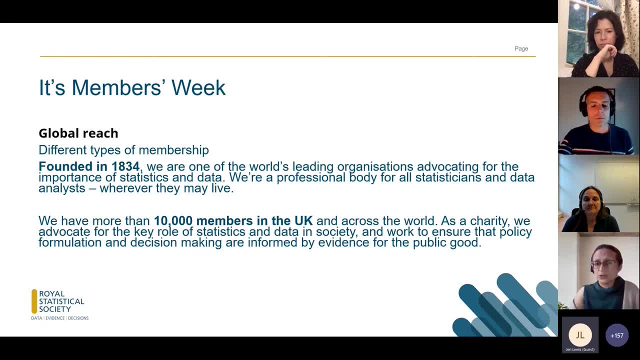 advocate statistics and data and society and work to ensure that policy formulation and decision making are informed by evidence for the public good. and this is, you know, has been crystallized during the current pandemic- the importance of having good statistics in driving local and global decision making. In addition, we have a different types of 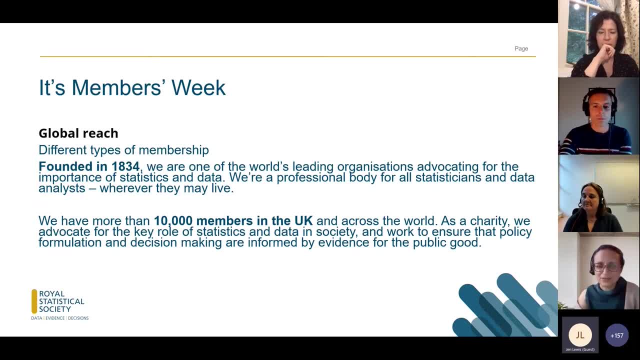 memberships as well. if you're interested and you're enticed after this session to join, join us, So please do. at the end of this presentation I'll as well share in the chat box the different links that you might want to. you know, if you're interested in the society to look at. 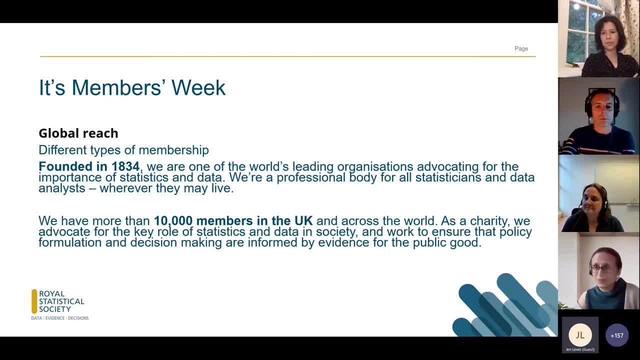 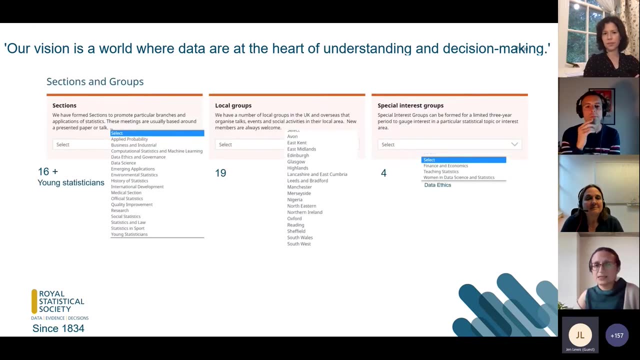 So wait for this space. I'll be presenting them in these slides, but wait for me to add them to the chat box because it might be easier for you to click on. Thank you, And so that's our vision is that our data is at the heart of understanding. 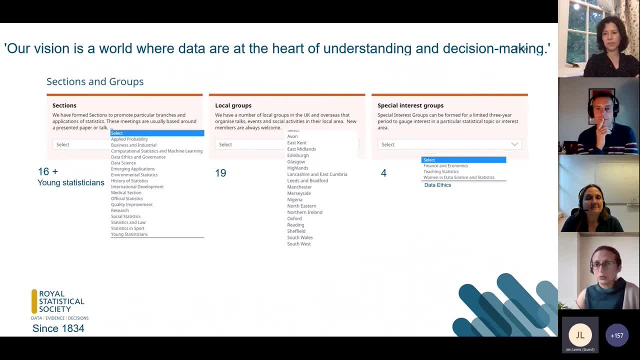 and decision making. We have a number of sections and local groups and special interest groups- A total of 16 sections, plus the young statisticians as well. specifically for young statisticians And within different localities, we have local groups that you know. come together and put 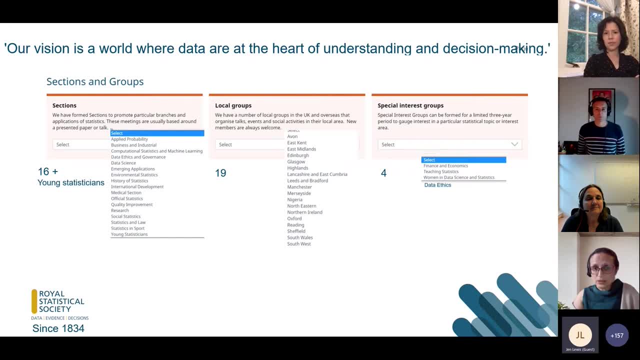 events as well. And some of these local groups are, you know, spread across the UK And some of them are even outside the UK, For example, the Nigeria local group. And then there are special interest groups, which is basically, you know, they haven't yet been sections, but people are. 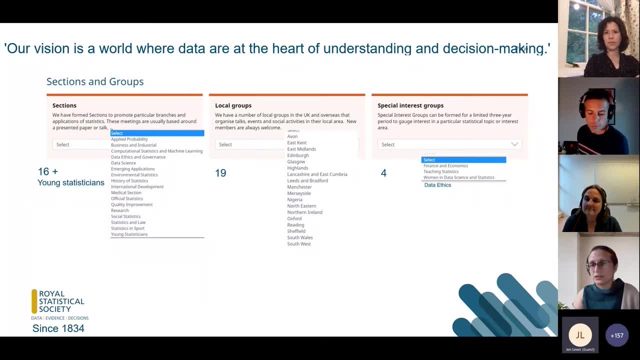 really interested in looking at trying to form a section including, for example, women in data science and statistics, data ethics and theory. Thank you, So that's the vision we see. Thank you, Thank you, Thank you, And I look forward to the future. 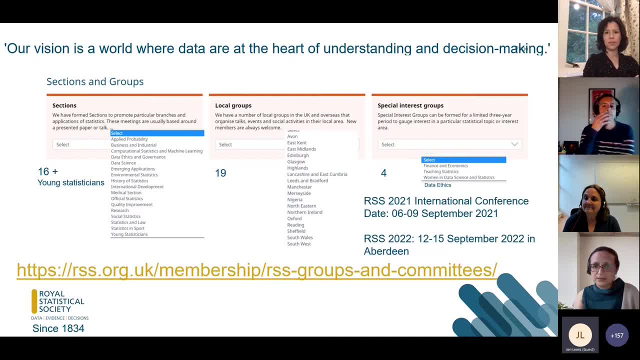 Thank you so much for joining us. Thank you And welcome to the panel. Thank you, Thank you, And it's great to have you all here. So we'll start with the first section here, which is the, and the upcoming one is in Aberdeen, 12 to 15 September 2022. 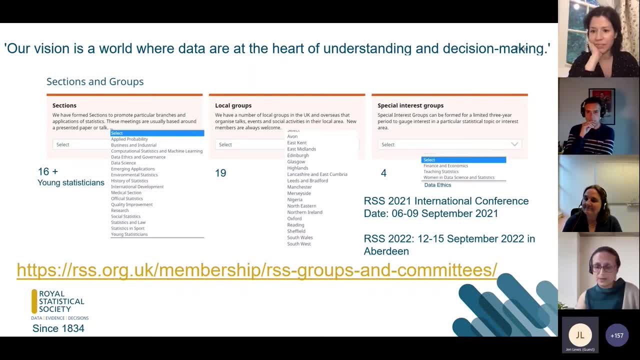 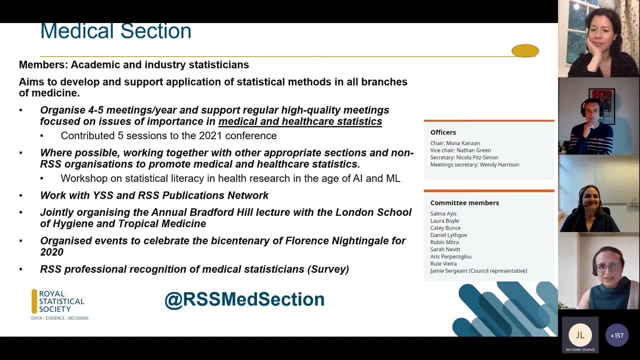 Our organiser, Ruth, will tell you a little bit more later about it. I hope so, Ruth. Okay, So I'll just briefly introduce the medical section which I chair, and this is basically the medical section aims to develop and support application of statistical methods. 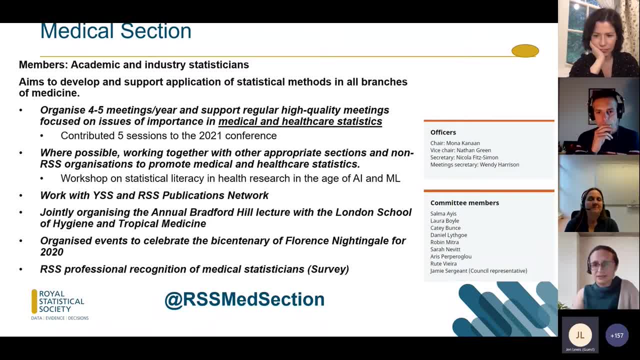 in all branches of medicine and, in fact, healthcare statistics, so any type of health data related that can inform decision-making. What we do is we organise four to five meetings per year- this one included, for example- and support high-quality meetings. 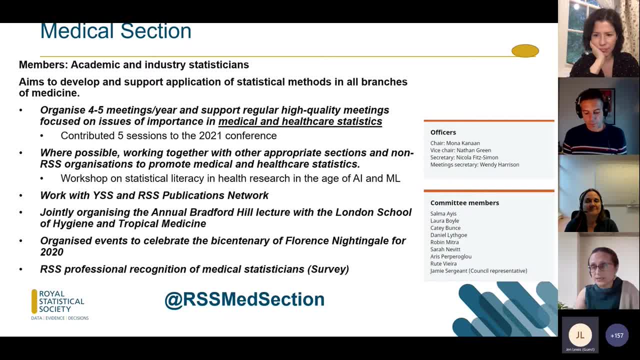 focused on issues of importance to medical and healthcare statistics. For example, we've contributed in the 2021 Conference 5 in the medical and healthcare statistics, we've contributed in the medical and healthcare statistics and we've also invited sessions to that conference. 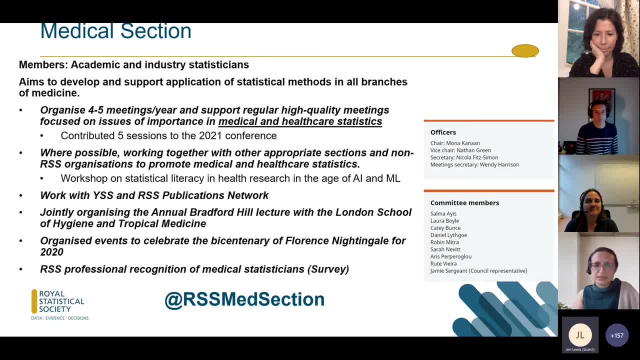 And these range from Bayesian inference to other as well, things like basically looking at reviewing the importance actually of acting as a reviewer, as a statistical reviewer, methodological reviewer for medical journals- And, in addition, where possible, we try to work with other appropriate sections and non-IQs. 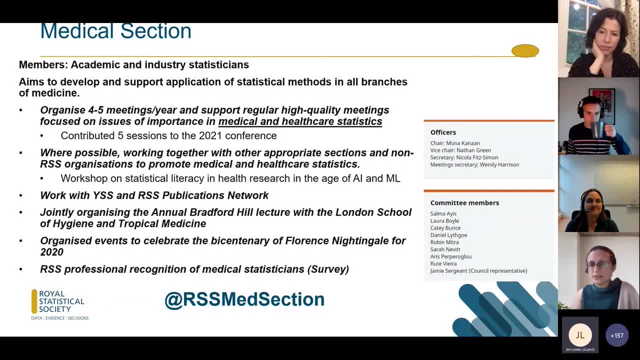 and we try to work with other appropriate sections and non-IQs, for example with RSS organisations, to promote medical and healthcare statistics. Our latest collaboration was with NIHR statistics group where we did a workshop on statistical literacy in health research in the age of artificial intelligence and machine learning. 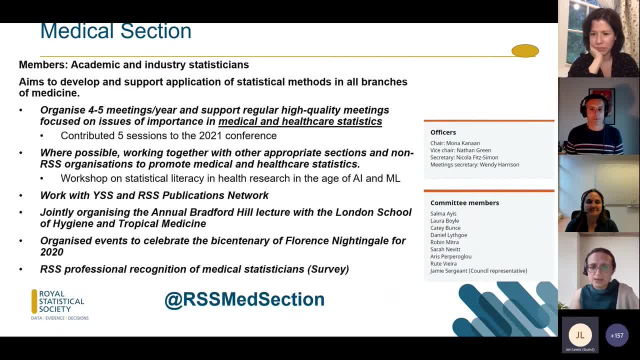 And as well, we have quite a bit of work with the Young Statisticians and RSS Publications Network. This is in addition to our joint effort with London School of Hygiene and Tropical Medicine Annual Bradford Hill Lecture. And we've done as well to celebrate. 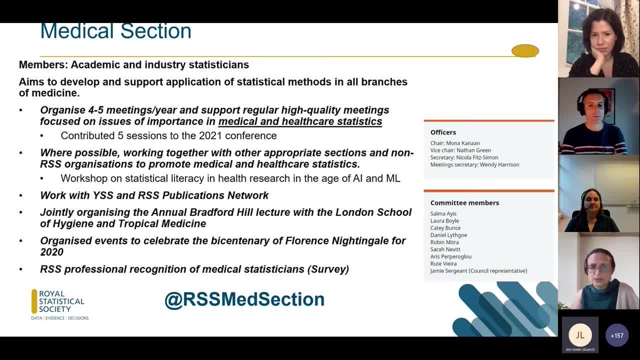 the bicentennial of Florence 19 in 2020.. We planned a number of events. Some of them went ahead in 2020 and some of them were postponed for later dates As well. we've been working. some of you might have received this survey. 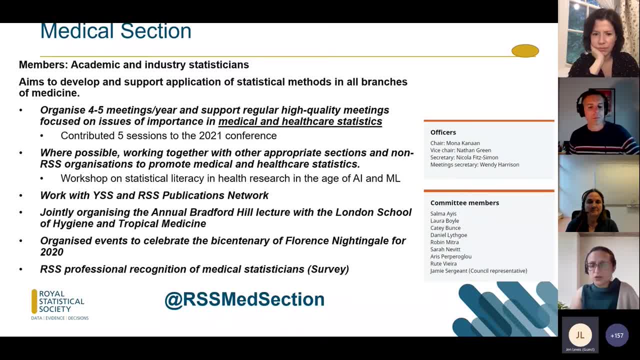 and contributed to this survey, which is the RSS Professional Recognition of Medical Statisticians. We're still working a bit more on the data and we'll probably share with you that when we finalise the analysis. In terms of officers, these are on the right-hand side. 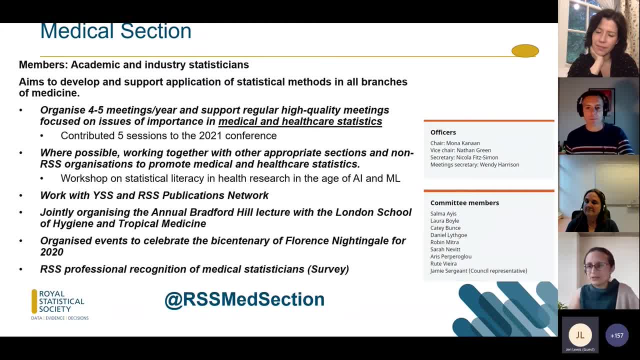 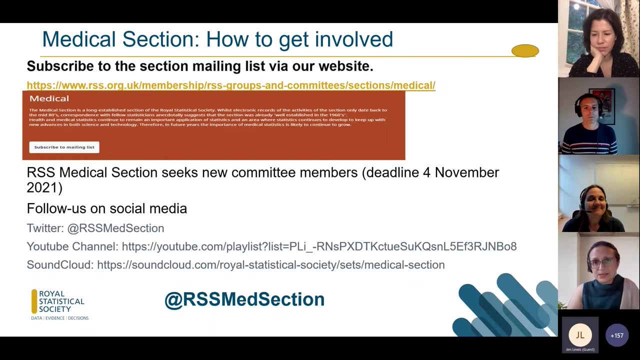 my right-hand side at least, basically, And you see we are a number of people coming together from across different walks. Okay, Now, if you're interested and if you think that's the medical section or RSS, some things that you'd be interested in contributing to. 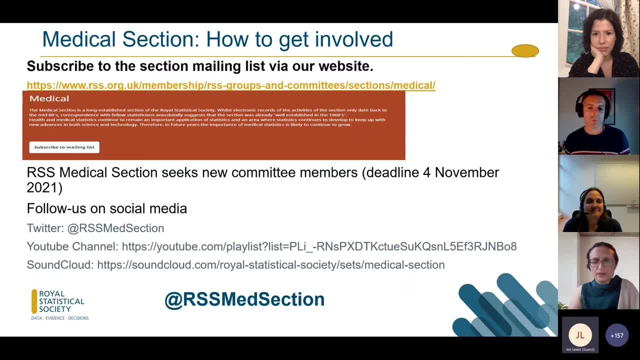 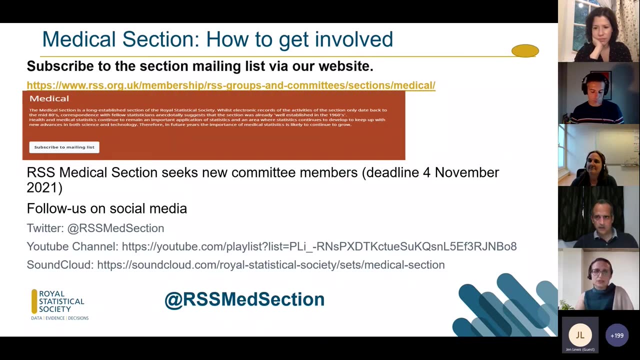 and as a nice form of discussion in terms of medical statistics, healthcare statistics and other types of statistical issues, please do look at our membership group and specifically the medical section. In addition, you can, if you're not simply interested in becoming a member, 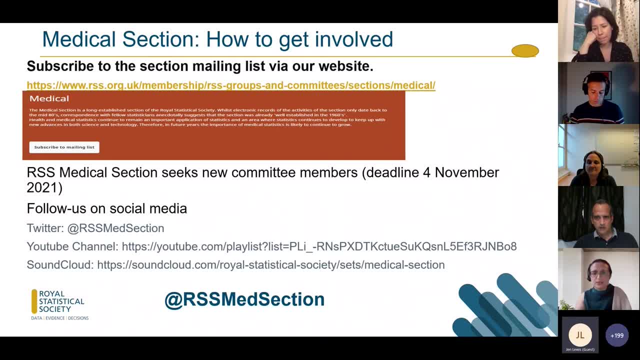 you can, however, subscribe to our mailing list, and here are the details of how you can do that. We are currently seeking new committee members and the deadline for this is next week, So please, if this makes you interested, please do put yourself forward. 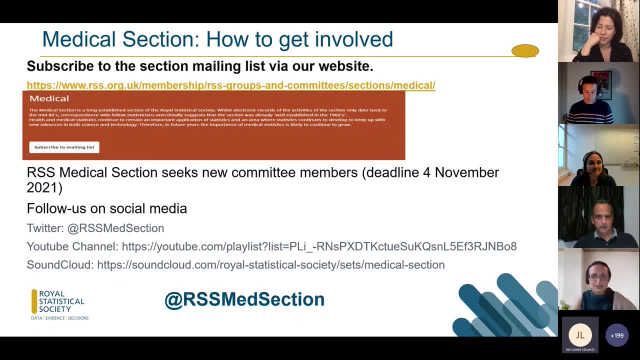 and you can follow us on social media- Twitter, YouTube and SoundCloud- where we have a number of, basically, presentations and podcasts related to the work we do. I think I'll stop here. Thank you very much for listening to the introduction of the RSS. 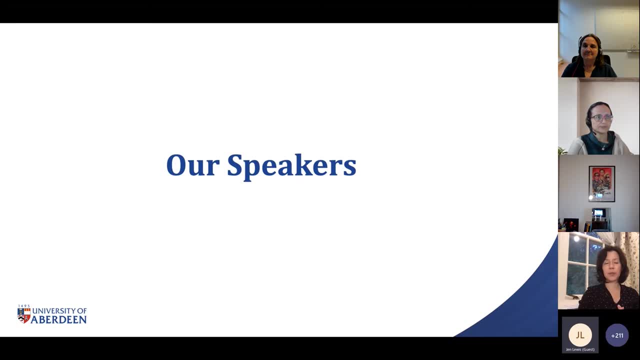 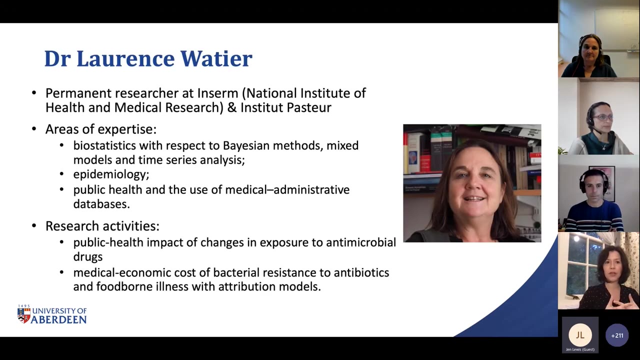 I'm actually delighted to introduce our speakers because they have quite a lot of experience in applying complex methods to time series, routine health data, And I will start by introducing Dr Laurence Wattier. So Laurence is a permanent researcher at the National Institute of Health and Medical Research. 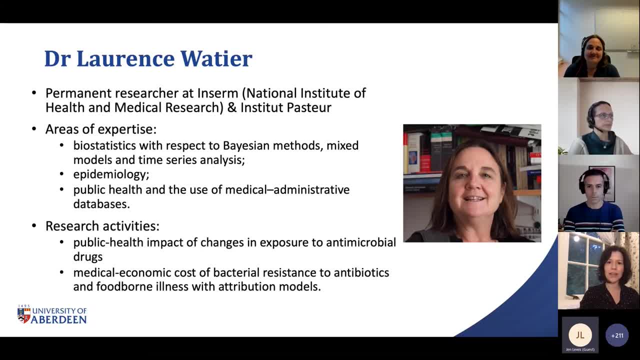 in France, also called INSERM, and also at the Institut Pasteur. So her areas of expertise are biostatistics with respect to Bayesian methods, mixed models and time series analysis. She has done a lot of work in epidemiology as well as public health. 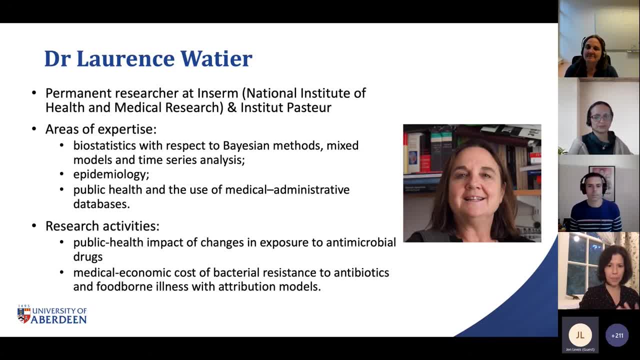 and the use of medical administrative databases. Her work recently has been focused on public health impact of changes in exposure to antimicrobial drugs and also on medical economic cost of bacterial resistance to antibiotics and foodborne illness, with attribution models And a very interesting fact about Laurence. 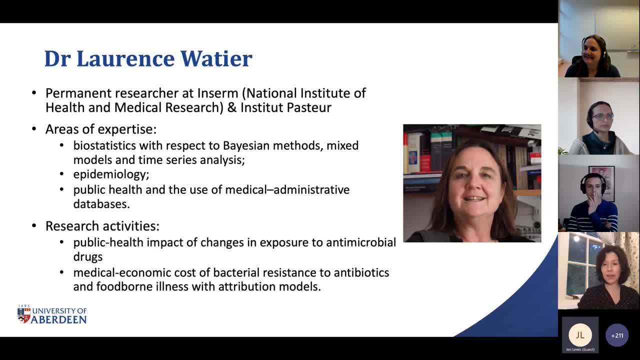 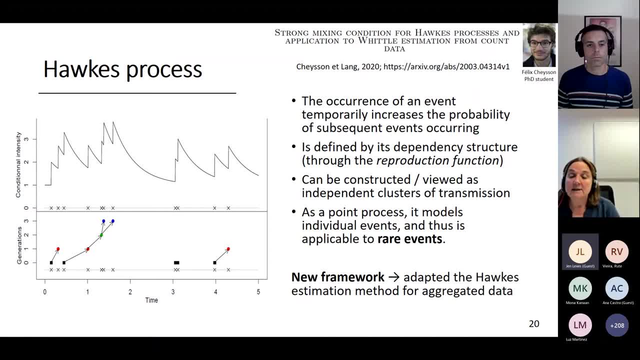 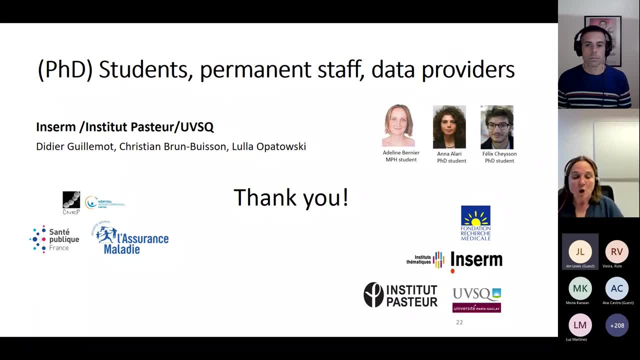 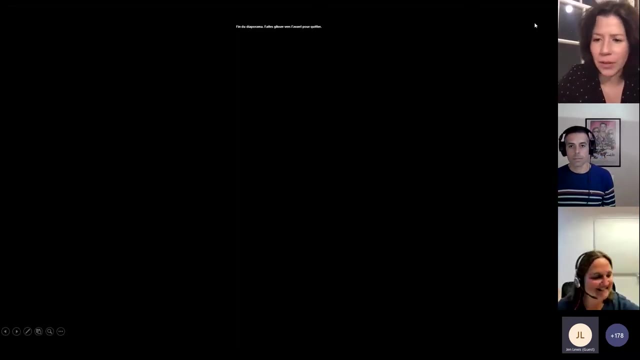 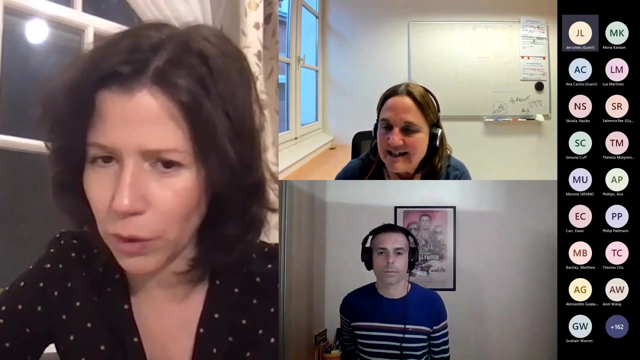 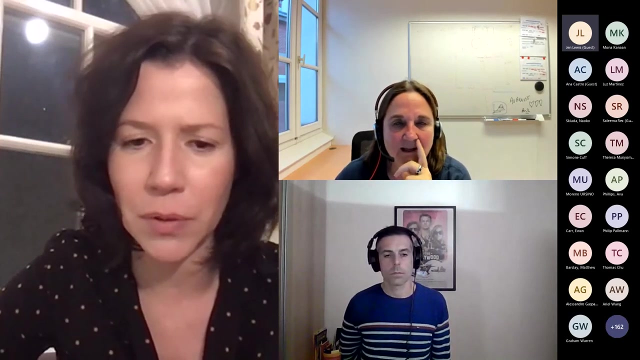 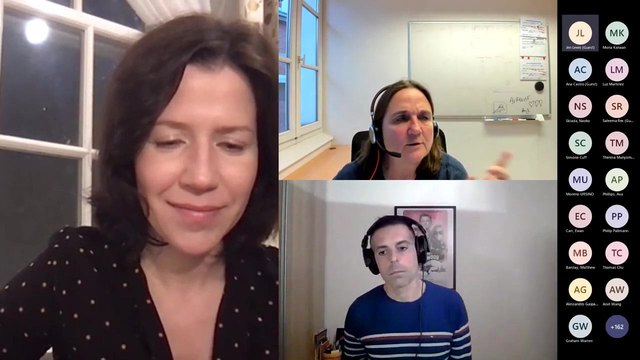 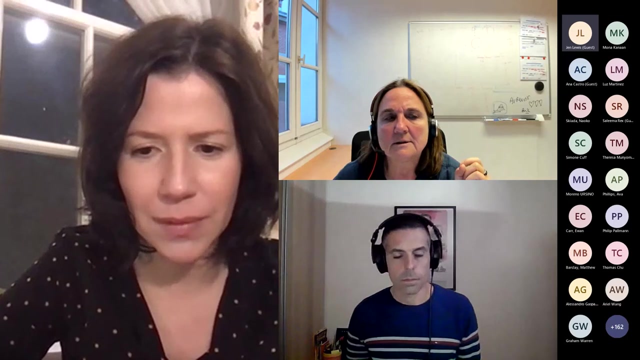 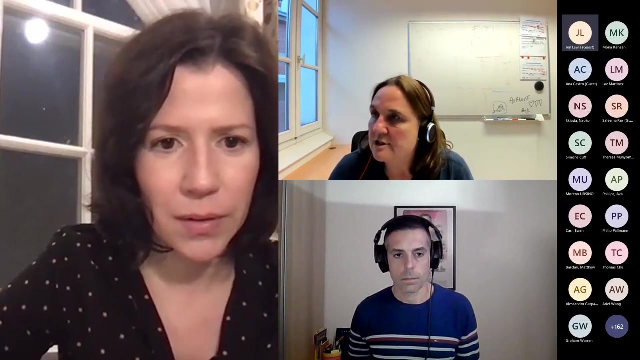 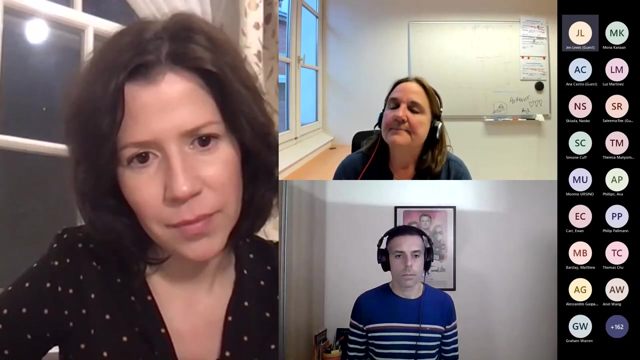 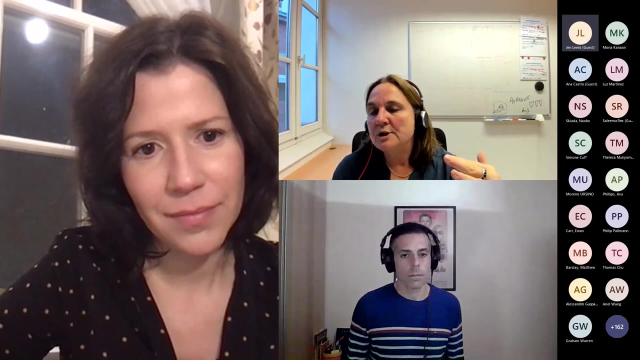 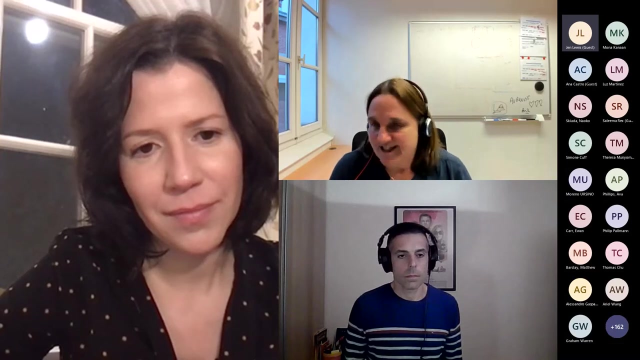 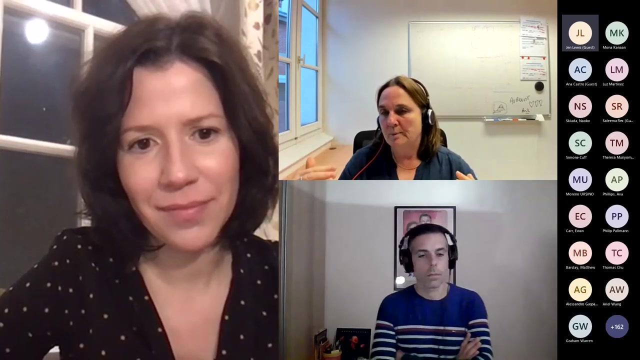 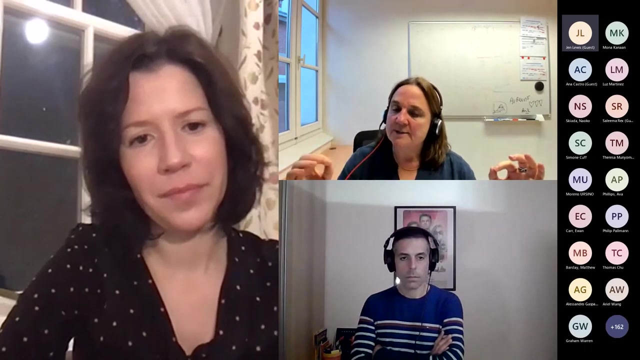 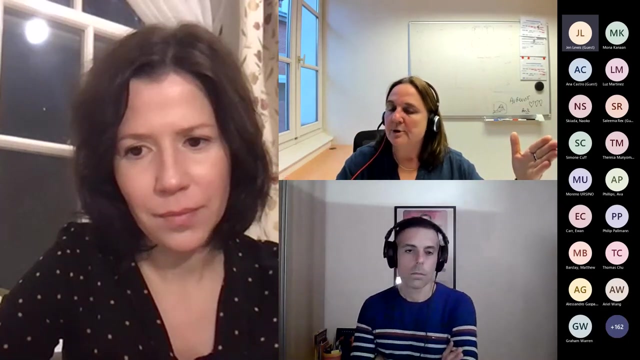 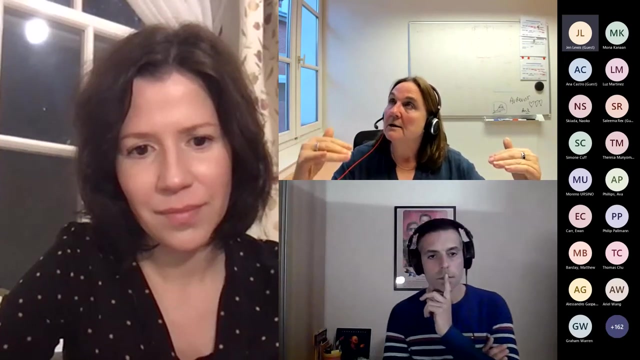 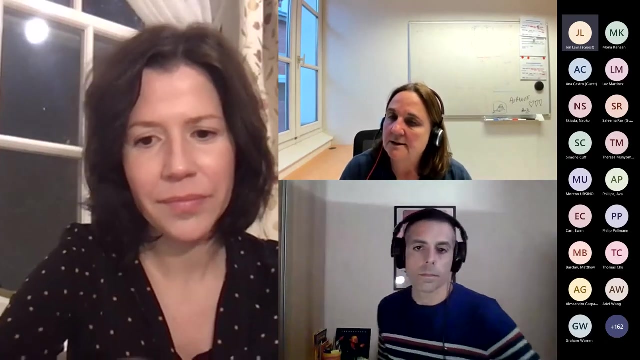 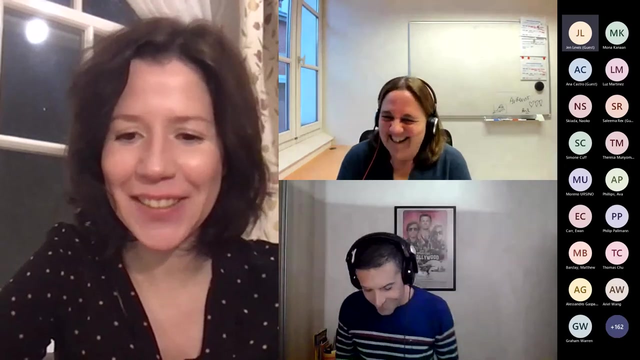 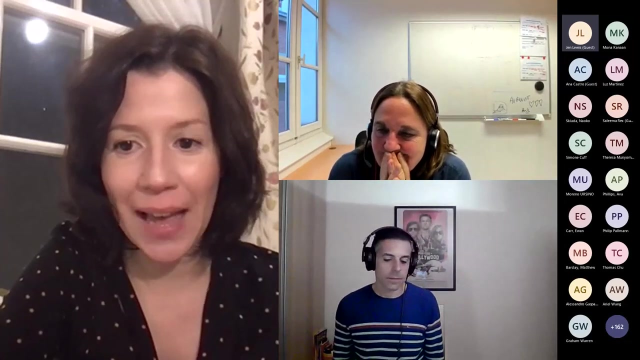 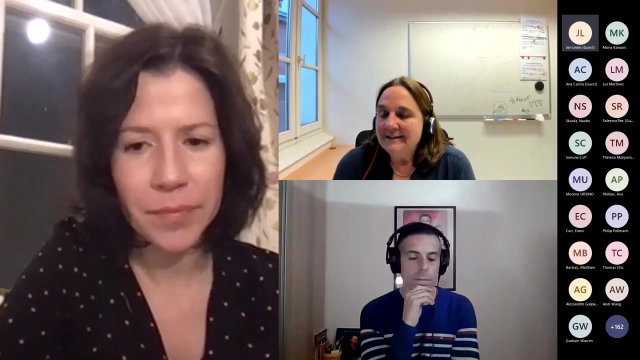 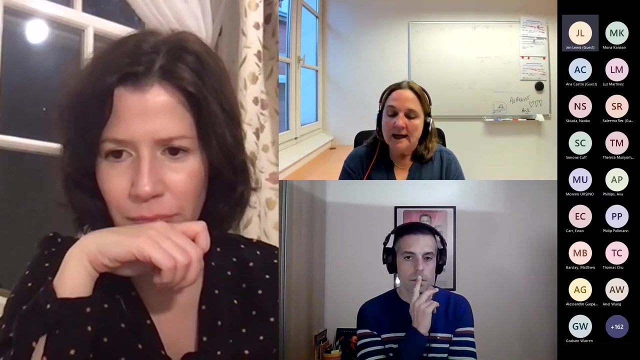 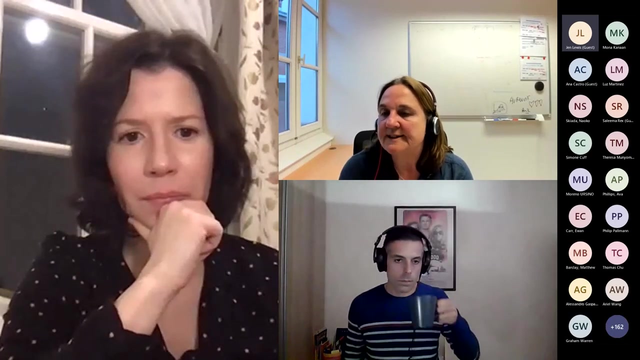 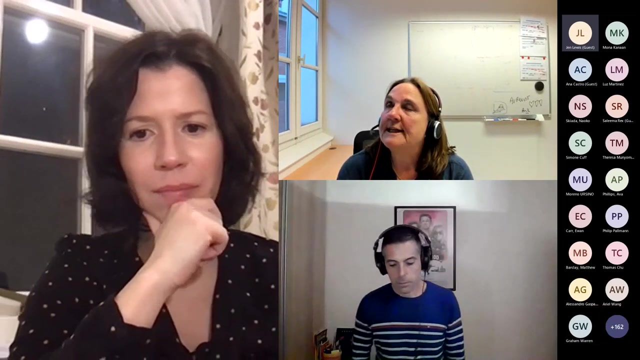 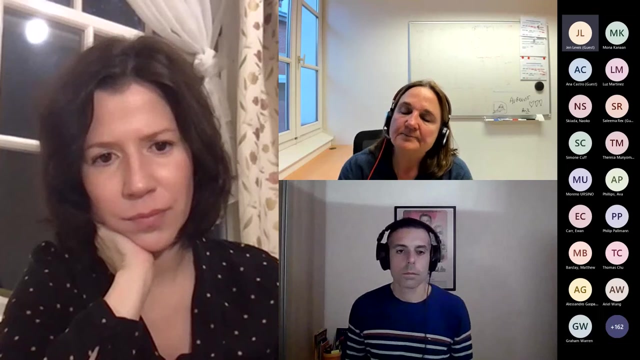 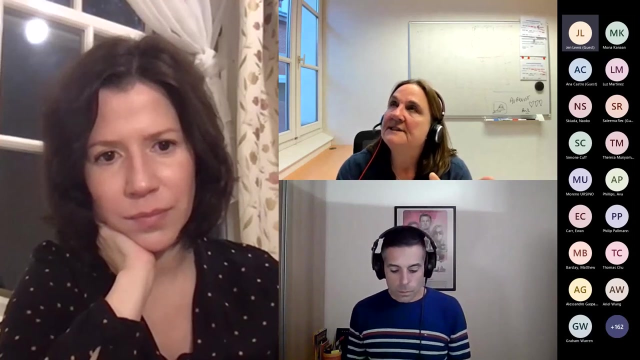 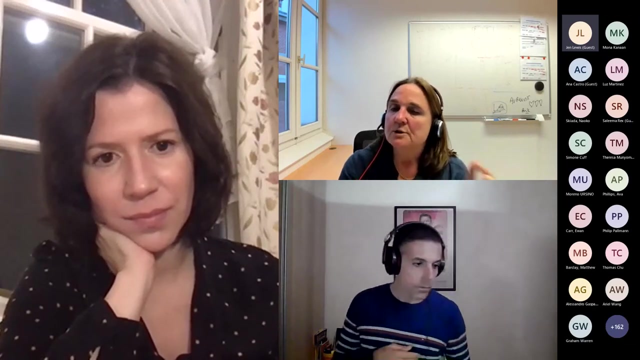 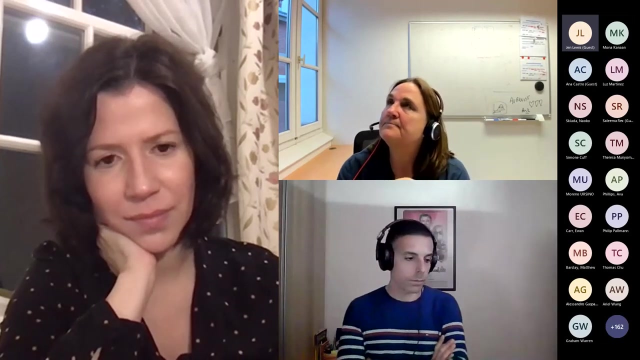 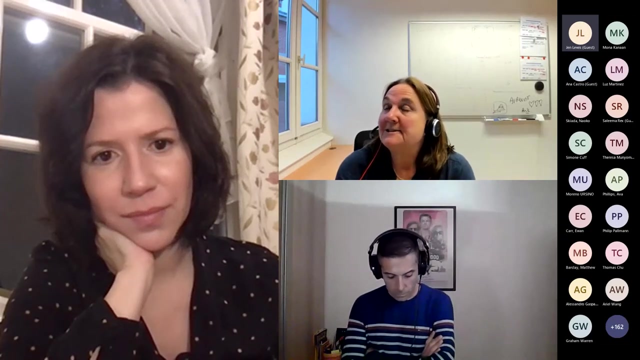 5., 6., 7., 8., 9., 10., 11., 12., 3.. I'm going to show you how to do it. I love you. Thank you for watching. Thank you, Thank you.